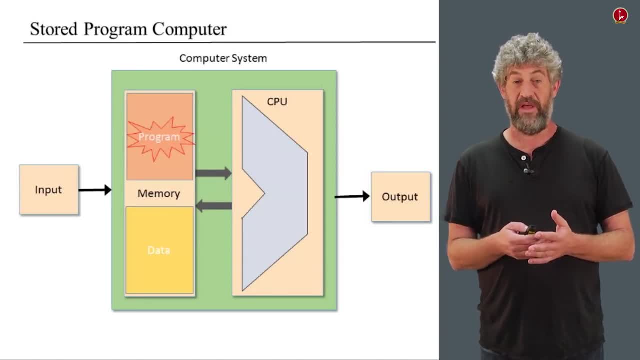 We're going to have a large piece of memory that's going to be used for two things: First of all, to store all the kind of the data that we're going to use in the computation. but, more interestingly, the memory will hold the program. 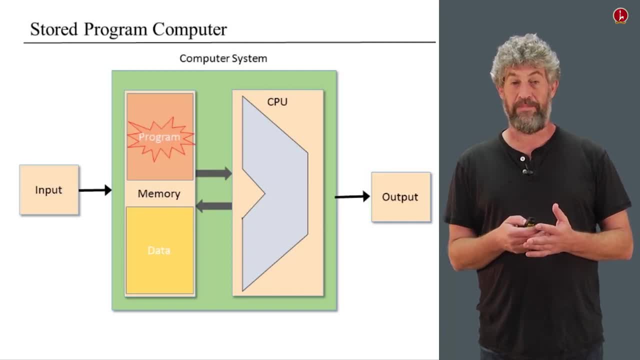 a sequence of instructions that are going to be executed one by one. Beyond that, we're going to have the central processing unit, which actually carries out these instructions And runs them and controls everything. So let us now look more closely how this actually happens. 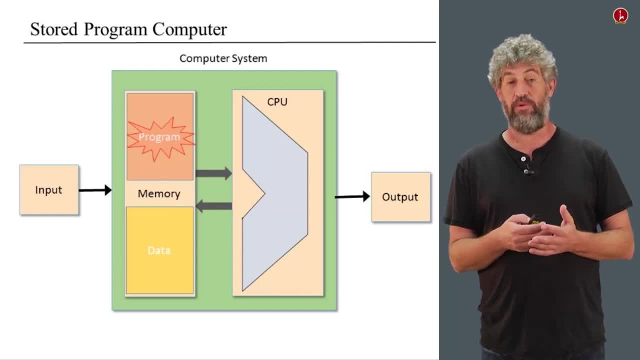 how the central processing unit is built and how does all the control back and forth work. And this is what we're going to describe in a general way- this unit- And later we'll actually talk much more specifically about the computers that we're building for this project. 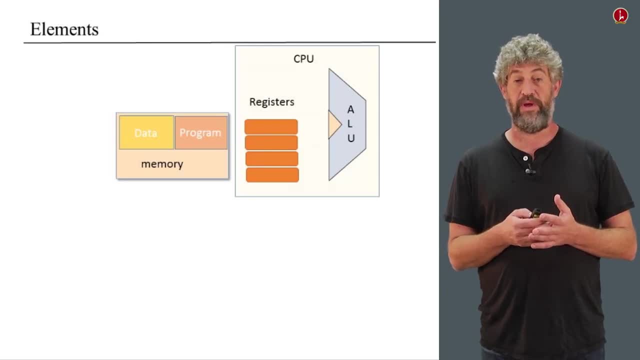 So, generally speaking, our compute, our CPU, is going to be composed of two main ingredients, two main components. One of them is what you often call the arithmetic logic unit. It's actually a piece of hardware that actually is able to add numbers. 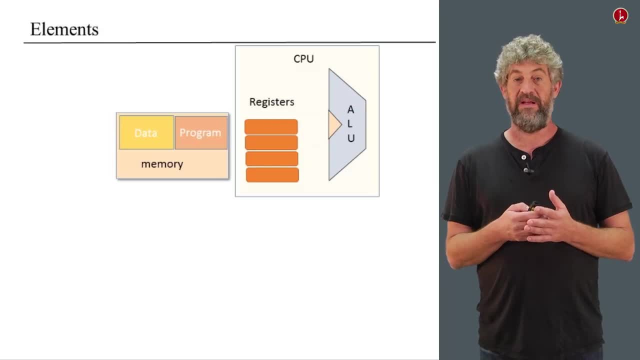 subtract numbers, maybe do logical operations and so on. The second element is there are going to be a bunch of registers, a bunch of places where we can store data, data that we're going to use for the rest of the computation. So this is going to be basically the core of the elements that the CPU is built of. 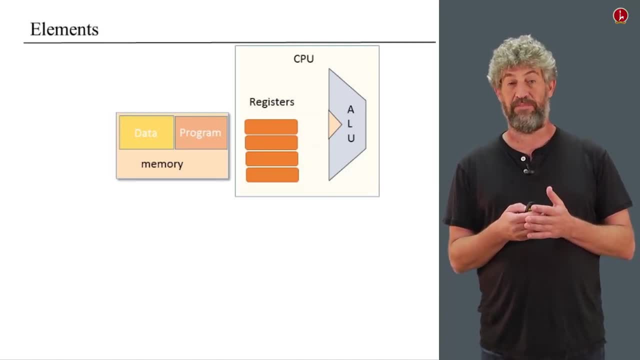 The memory itself, as we said, has two parts: The part that stores the program and the part that stores the data. To try to understand how all these things work together, it's best to actually consider the flow of data. what kind of information needs to pass within the computers from side to side? 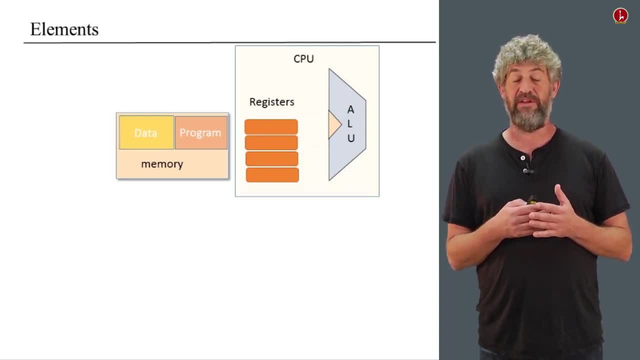 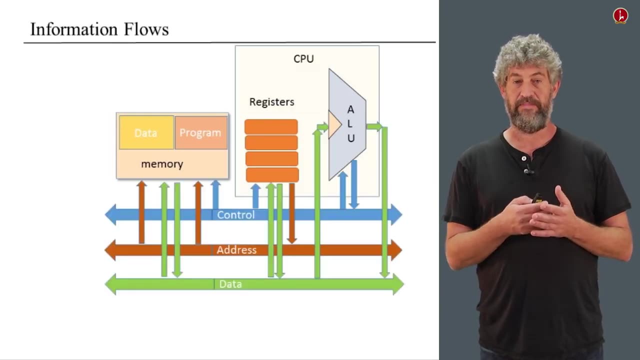 And this is what we're going to actually now try to do- try to describe the various pieces of information that go from side to side in this computer and how we control them. So basically, there are, I would say, three types of information that usually 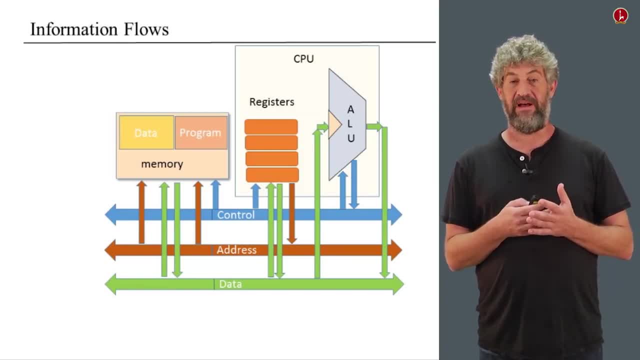 pass throughout the system, And one of them is the data. When we have numbers that need to be added, of course the numbers needs to be moved from some from one place to another, from the data, a memory, to the registers, to the actually arithmetic logic unit, that's. 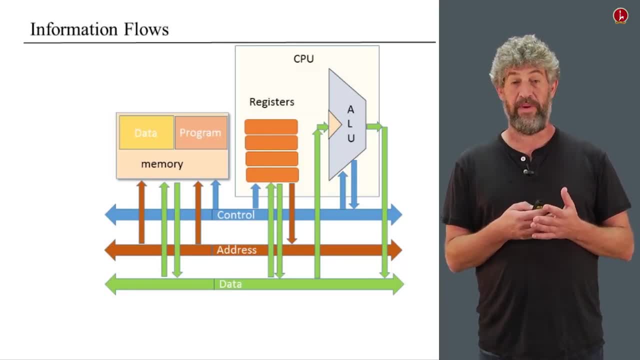 going to do something with them and back. The second type of information that we need to control is what's called addresses. What instruction are we actually executing now? What piece of data within the memory do we need to access now? These are in addresses. 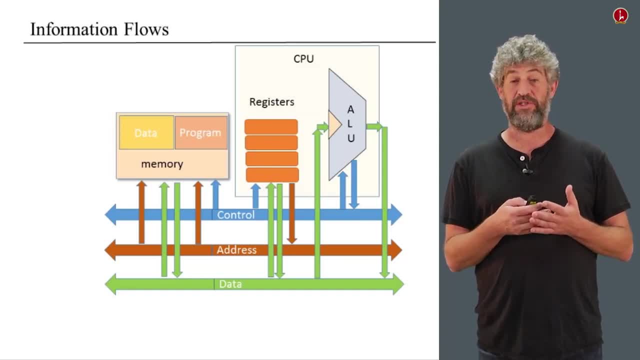 And, of course, there's going to be a, there is going to need to be a big bunch of wires that actually do all the control, that actually tell each part of the system what to do at this particular point, And this is called the control. 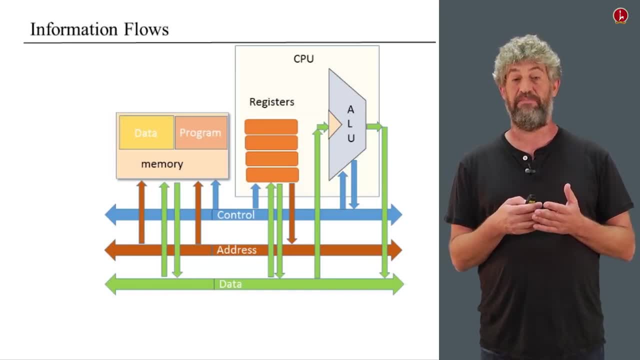 Sometimes all these three pieces of the, each one of these pieces of information is actually going to be implemented by wires, by a set of wires, sometimes called a bus. So we're going to have in a typical system computer, we're going to have a data bus, an address bus. 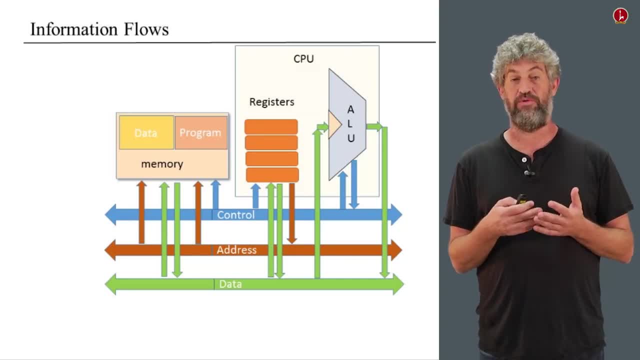 And sometimes the control bits are called the control bus, sometimes they're just called control wires. So let's look at the different pieces that we have in our computer and see exactly what kind of information they get and emit. Let us start with arithmetic logic unit. 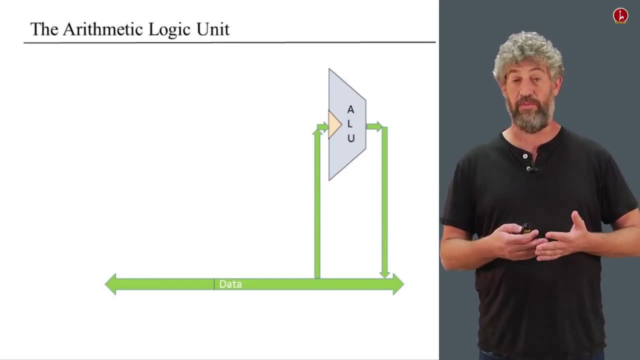 This is the conceptually the simplest and clearest part of the CP of our computer. It basically needs to be able to accept numbers and add them, subtract them, do some logical operations on them. So it's very simple. We need simply need to have some information from the data bus. 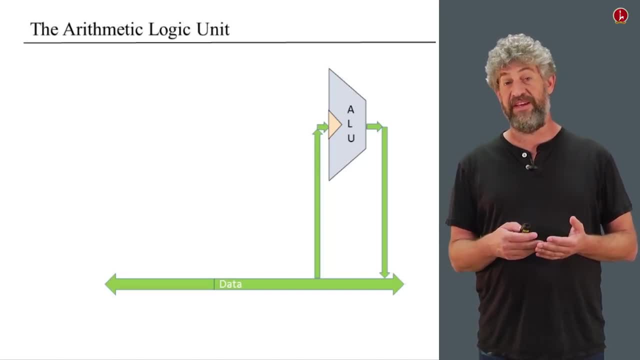 connecting to the LU and then information and then feed the output of the LU back into the data bus. That's going to be a and from there, of course, it's going to have to go to other places that also connect to the data bus, like the memory or the registers. 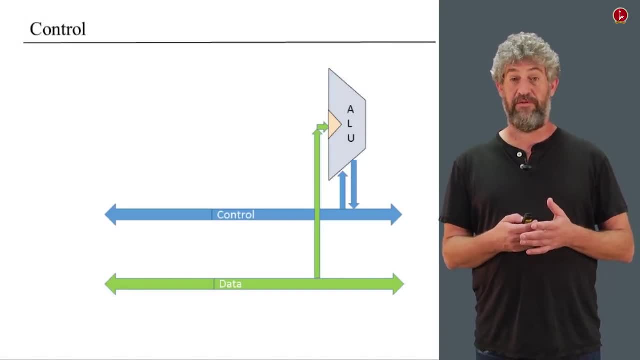 There's one other piece of info, but other type of piece of information, that the ALD would ALU- will need to be connected to. This is the control bus. On one hand, of course, the ALU needs to know what kind of operation it does it. 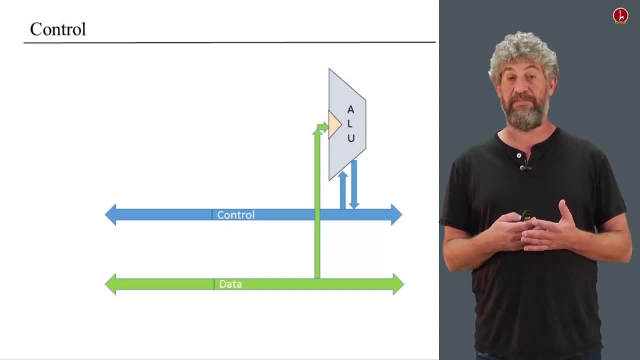 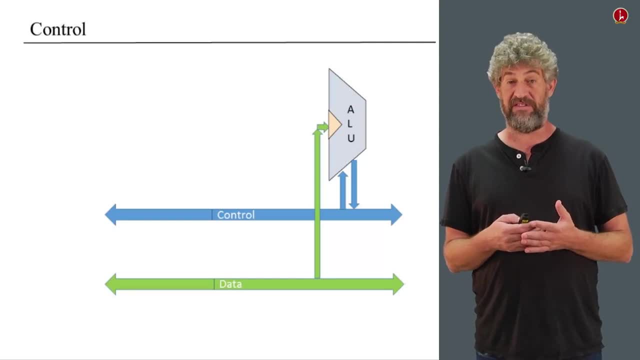 it's going to be able to have to be able to tell the other parts of the system what to do, For example, if it sees that a certain number is greater than zero, that could control the jump in the next instruction, what the next instruction will be. 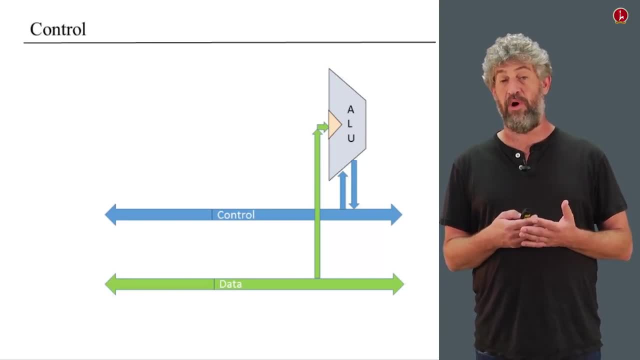 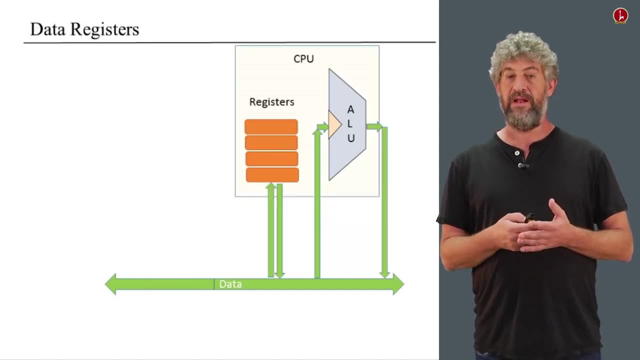 This control will happen through the control bits, So we're going to also have to get, take some information from the ALU and feed it back to control the rest of the system. Let us consider now with the registers. The registers, conceptually, are very simple. 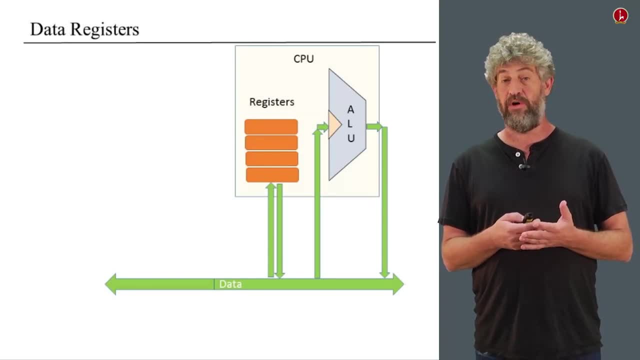 Again, we store intermediate results in the registers, So we're going to be have to be able to take data in from the data bus into the registers And then also take data from the registers and feed them back into the data bus. 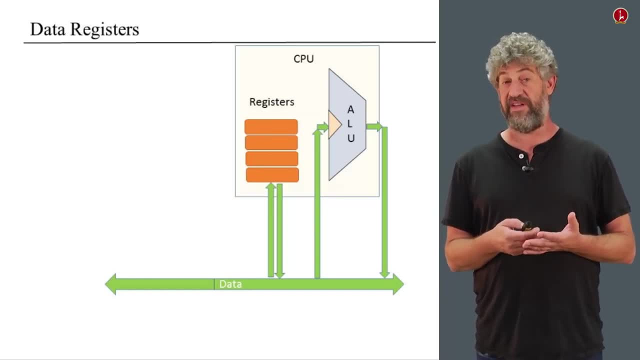 And, of course, where would they go, from the data bus To other parts of the system, such as the ALU. So this is the first thing, that of course, we will have to connect all the registers to the data bus. The second piece of information is sometimes, as we've discussed previously, 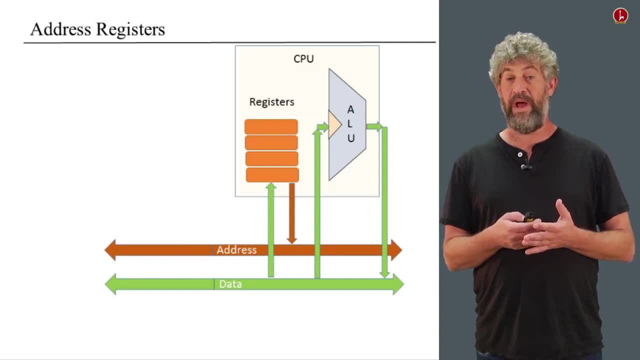 we. some registers are used to specify addresses, The way we actually achieve indirect addressing into a RAM or jump into a ROM address. the way we do it is usually we put numbers, addresses into a register and then that specifies where we want to access. 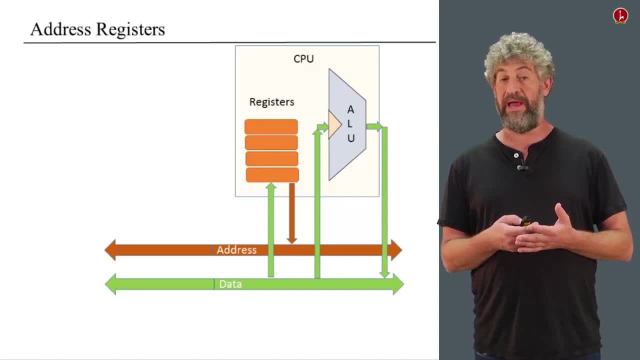 So we're going to also have to have registers control a connected to the address bus, which controls again the memories, that which actually then feeds into the memory. So that's the second type of information we'll need to have. We will have to have some registers that are address registers, either exclusively or 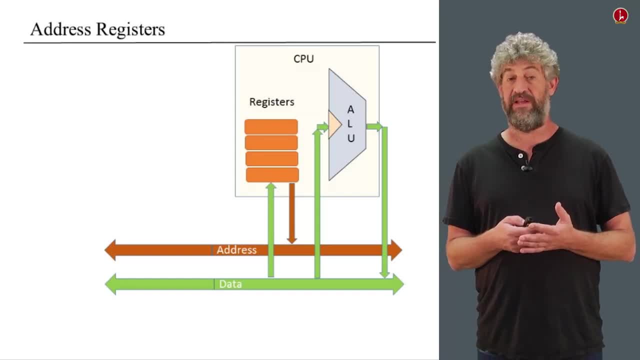 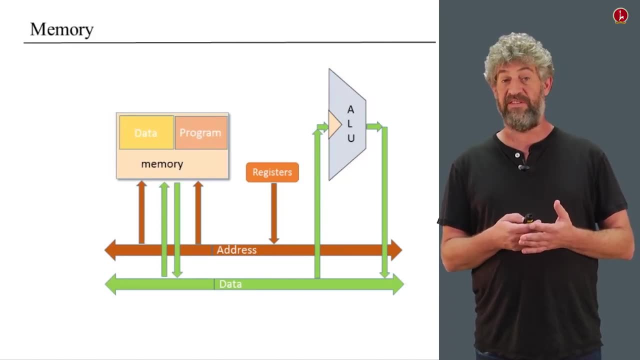 both address and data registers, and these will need to feed into the address bus. The last piece of info, the last piece that we need to talk about, is the memory. So, on one hand, the memory needs. we always need to specify what. 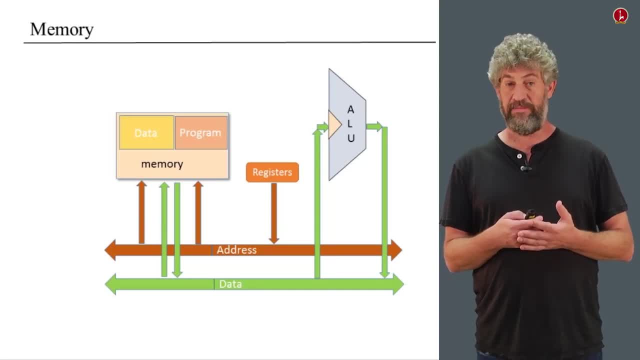 address of the memory are we going to be working with And specified, of course, by the address bus. That's the whole point And, of course, once we actually work with a certain address, we're going to be need to be able to read it or write into it. 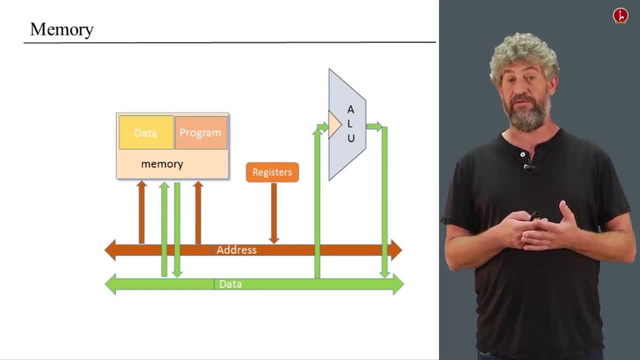 Get information from it or or put information into it. So, of course, the data, the input and the output of the memory unit will have to be connected to the, to the data bus. Let us look slightly more clo closer inside. 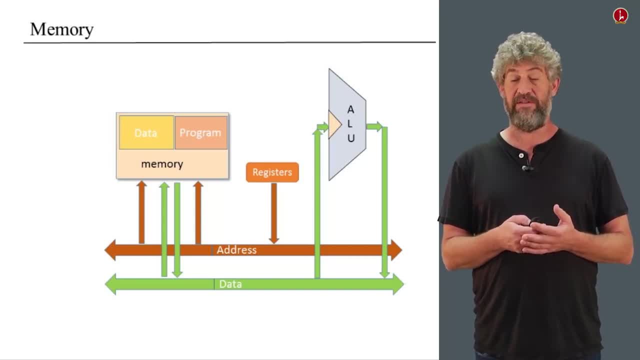 There. there are two pieces to the memory. There is a data memory and there is a program memory. Let's a talk a little bit about each part of these. Looking at the data memory, that where it's going to need to get an address of a data piece that needs to be operated upon.